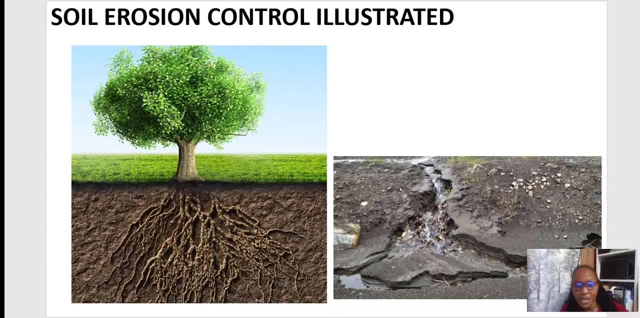 And then also you see the grasses, which significantly play a bigger role, even than the forest, in terms of reducing soil erosion. The next picture there showcases bare land where the levels of soil erosion are very high. You can see it's a picture showcasing a rainy season and there are actually significant soil erosion that can be seen. 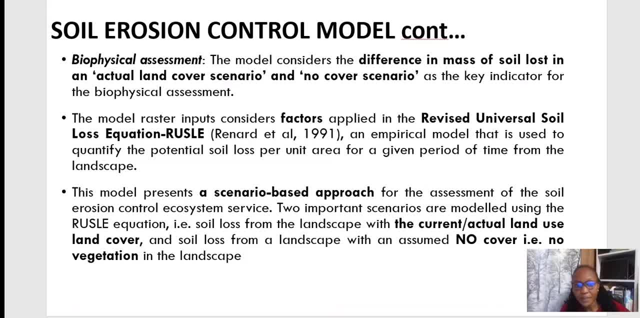 You can see, it's a picture showcasing a rainy season and there are actually significant soil erosion that can be seen. So what are the biophysical assessment or biophysical indicators that we need to consider when it comes to the soil erosion control model? The model considers differences in mass of soil lost in an actual land cover scenario and a no cover scenario. 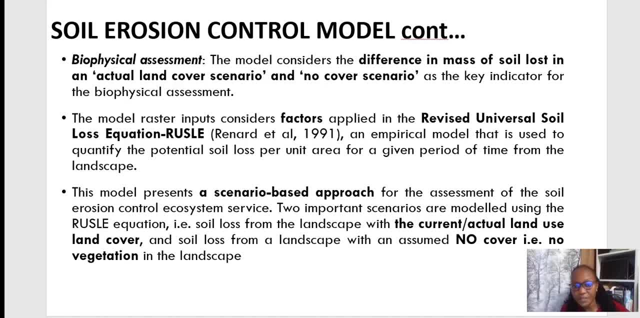 Remember we said, the color tool basically is built based on degradation aspects and that's why comparing the two scenarios is very key And therefore this forms the key indicator for the biophysical assessment. The model RASTA input considers factors applied in the revised universal soil loss equation RASO. 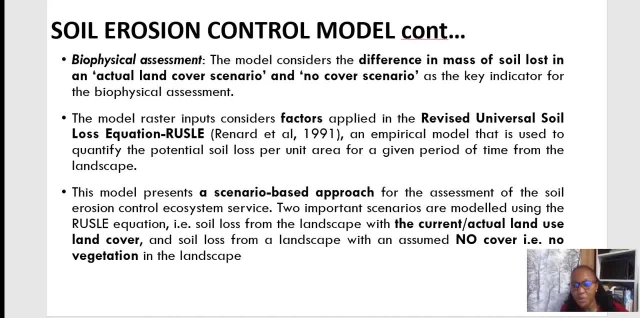 I'm sure most of you are familiar with this equation. It's an empirical model that is used to quantify the potential soil loss per unit area for a given period of time from the landscape. The model presents a scenario-based approach for the assessment of the soil erosion control ecosystem service. 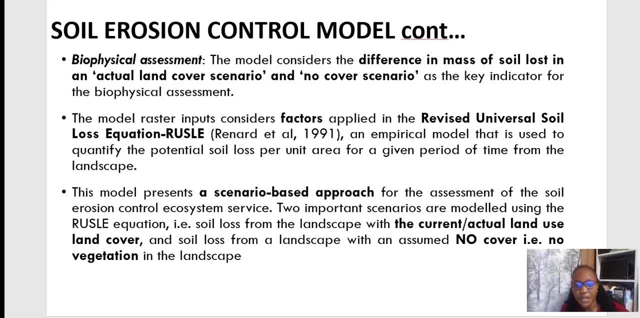 Two important scenarios are modeled using the RASO equation, For example. what we mean in this case is that soil loss from the landscape with the current or actual land use land cover and the soil loss from the landscape with an assumed no cover or no vegetation in the landscape. 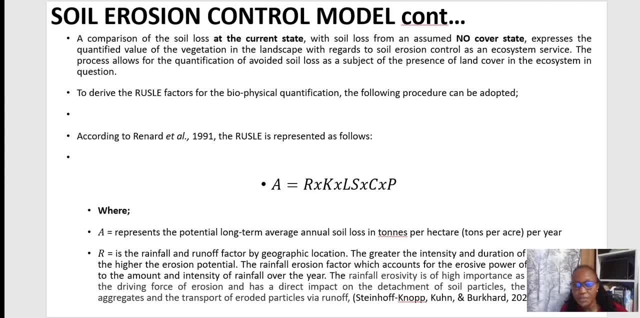 Therefore, a comparison of the current state with soil loss from an assumed no cover state expresses the quantified value of the vegetation in the landscape. with regard to soil erosion control as an ecosystem service, The process therefore allows for quantification of avoided soil loss as a subject of the presence of land cover in the ecosystem in question. 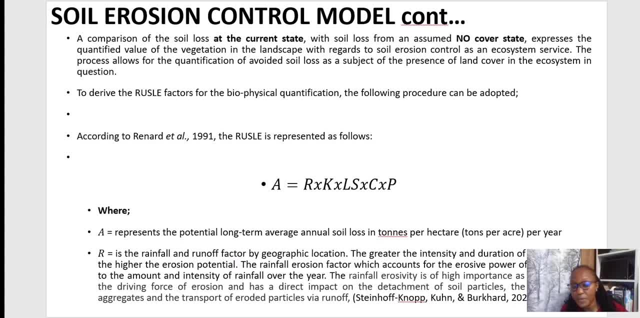 To derive the RASO factors for the biophysical quantification. the following procedure continues: The following procedure continues. In this particular case, the model presents the RASO equation as it is showcased here. The R is the rainfall and runoff factor by geographic location. 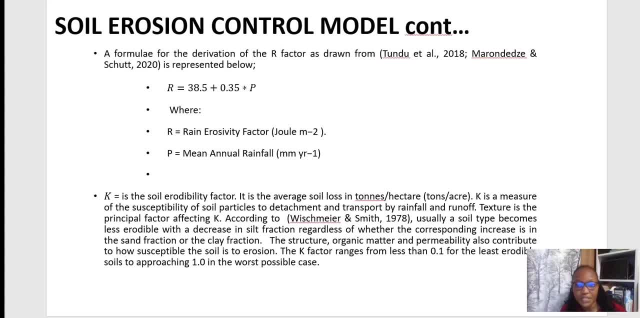 A formula for the derivation of the R factor has been presented. You can be able to visualize it. Those that have had an opportunity to work with the RASO equation, I'm sure, are familiar with these factors. The K is the soil. 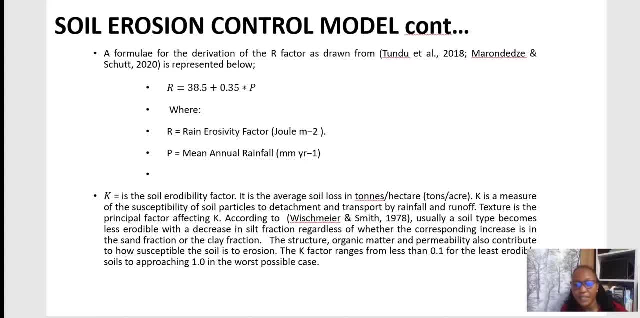 erodibility factor. It is average soil loss in tons per hectare. It's a measure of sustainability of soil particles to detachment and transport by rainfall and runoff. Texture is a principal factor affecting K. According to Wittner and Smith in 1978, soil type becomes less erodible. 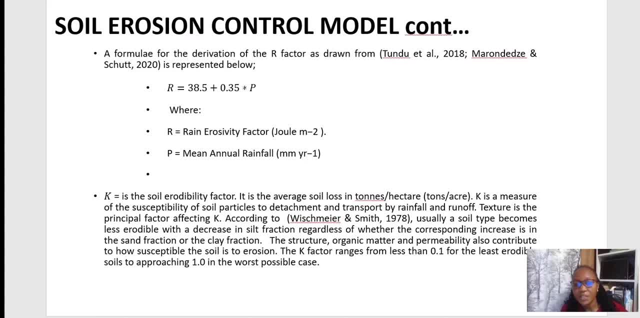 with a decrease in silt fraction, regardless of whether the corresponding increase in the sand fraction or the clay fraction. I do not want to get into the details of the extraction of these factors, but this information has already been provided for in the guide for you to be able to. 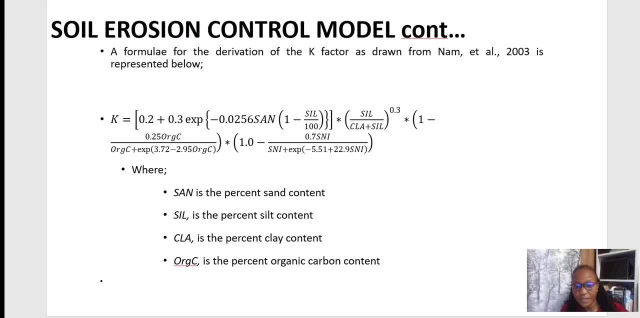 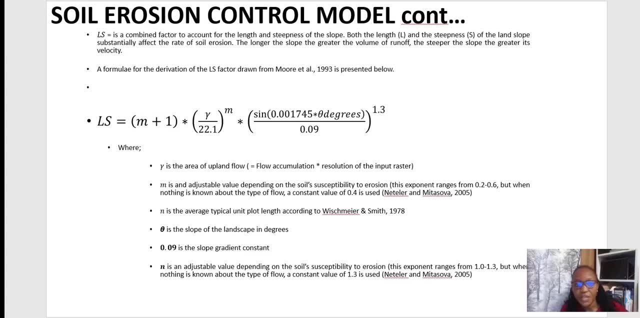 follow up and know how to either silt clay and sand. That is what determines the K factor and the erodibility of the soils. And then the LS factor is a combined factor to account for the length and the steepness of the slope. Both the length and the steepness of the land slopes are. sustainability factors, And then the LS factor is a combined factor to account for the length and the steepness of the soil. And then the LS factor is a combined factor to account for the length and the steepness of the soil, And then the LS factor is a combined factor to account for the length and 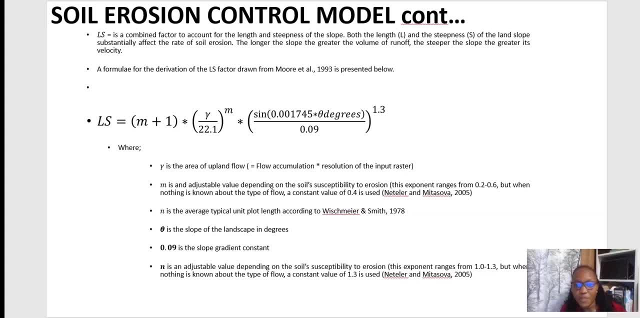 The longer the slope, the greater the volume of runoff. The steeper the slope, the greater the velocity. A formula for the extraction of the LS has been displayed there And you can actually follow up in the Callwood tool guide to be able to know how to extract the LS factor. 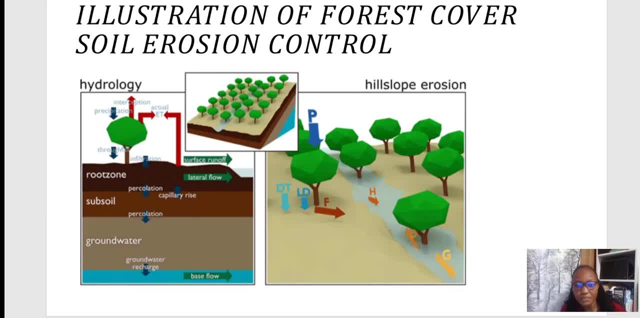 An illustration of the forest cover. soil erosion control has been demonstrated there. Like I said, grass plays a bigger role compared to forest, But because we'll be running the forest part of the models, the submodel- within the soil erosion control, I felt it's. 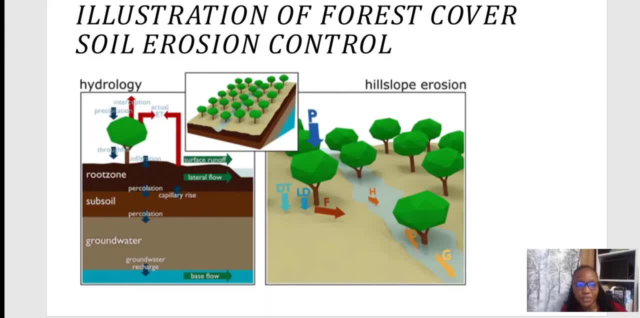 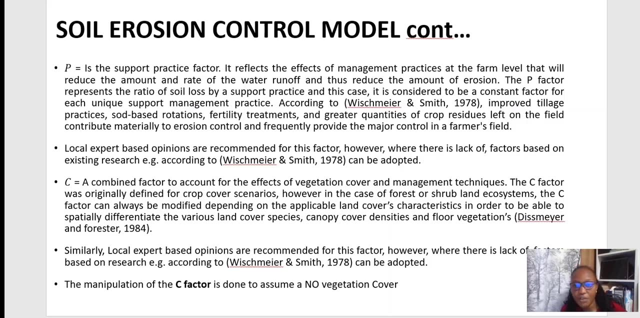 good to just look at how the root zone enable the population of the water and therefore slow down the movement of water and in that case also slowing down any soil erosion that could have taken place. Further, the P factor is a support practice factor. It reflects the effect of management practices at the farm level that reduce the amount and 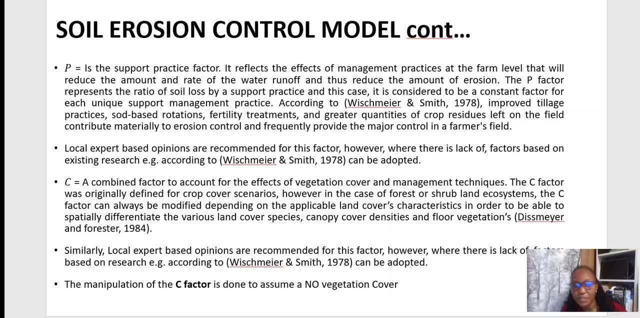 the rate of water runoff and thus reduce the amount of erosion. The P factor represents the ratio of soil loss by support practices, and this is considered to be a constant factor for each unique support management practice, For example, improved tillage, soil-based rotations, fertility treatment and greater 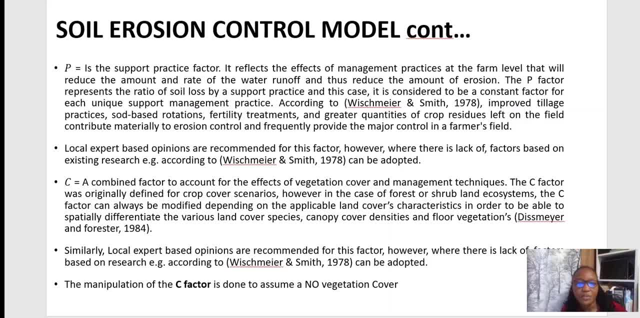 quantities of crop residue left in the field are known to reduce actually soil erosion and frequently provide the major control in farmers' fields. And then we have the C factor. It's a combined factor to account for the effects of vegetation cover and management practices, and this is where the forest, the shrubland, the grassland ecosystem come in. 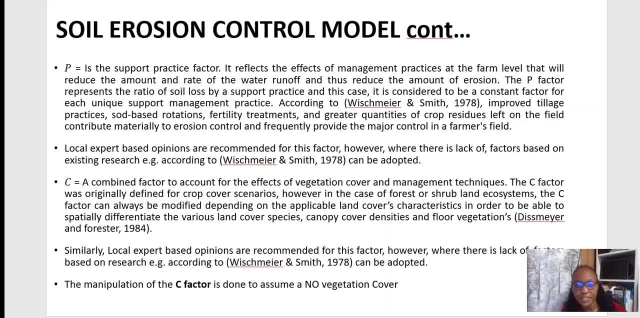 And therefore they are modified depending on the applicable land cover characteristics in order to be able to spatially differentiate the various land cover species and canopy cover densities and flow vegetation, and in the ability to actually slow down soil erosion. So here it is where, in the model, we are manipulating the C factor because we have said it's a. 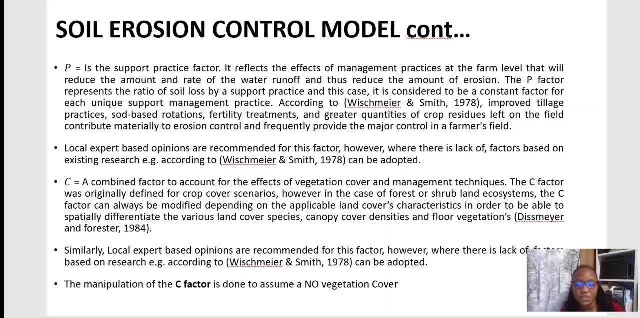 scenario-based approach, where we manipulate the C factor and have a no-vegetation cover to be able to visualize under cover and a no-cover vegetation. how much soil are we likely to be avoiding in terms of loss, so that we can be able to model and actualize the value? 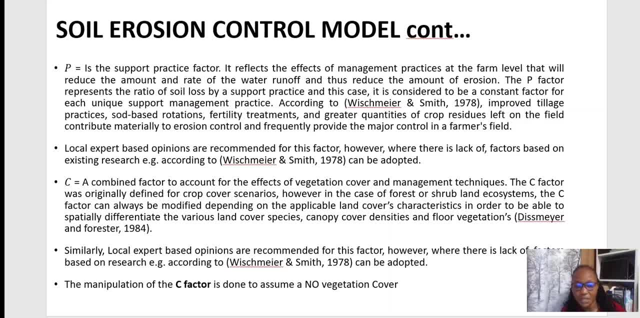 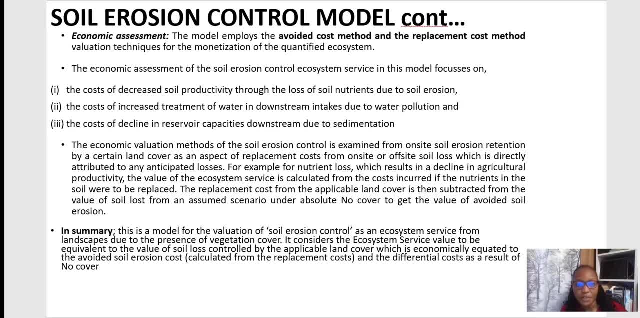 that would accrue to forest or rangelands. that means shrublands and grasslands. For the soil erosion control model, when you look at the economic assessment, it's the avoided cost method and the replacement cost method which are valuation techniques. 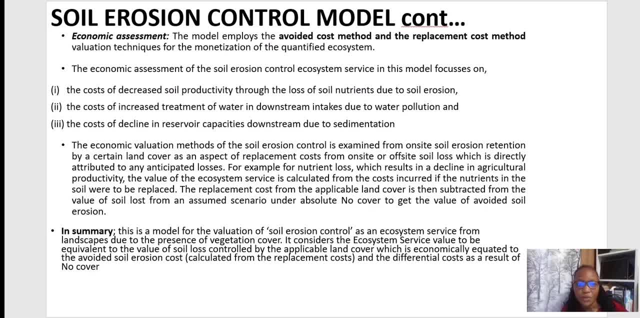 for the monetization of the quantified ecosystem. So when we look at the economic assessment of soil erosion control service, in this model we focus on the cost of decreased soil productivity through the loss of soil nutrients. Number two: we look at the increased treatment of water in downstream as a result of water. 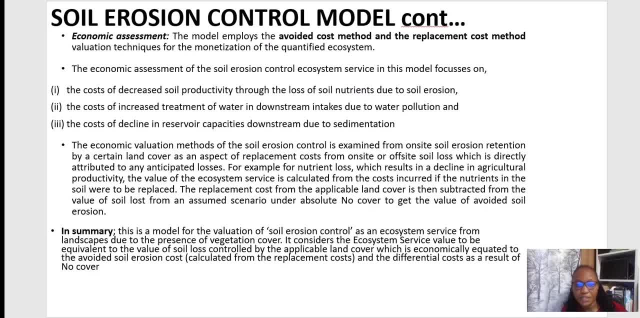 pollution and, in most cases, the levels of sedimentation. We thirdly look at the decline in reservoir capacities as a result of sedimentation. Remember we said, when we look at the water storage, when we look at flood control capabilities, we are looking at declining reservoir capacities to hold enough water as a result of sedimentation. 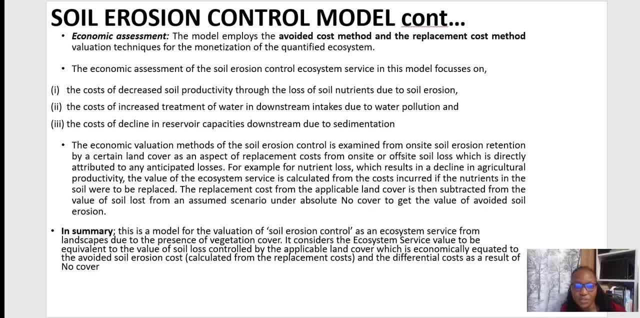 These are some of the factors that we are also looking at under soil erosion control model. The economic valuation methods of the soil erosion control, therefore, is examined from an on-site erosion retention by a certain land cover as an aspect of replacement cost from on-site or off-site soil loss which is directly attributed to any 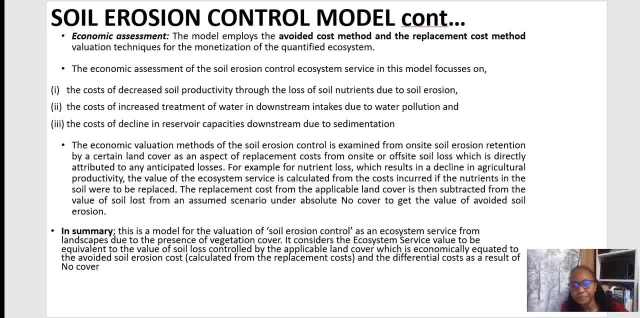 undisciplined soil erosion, For example, nutrients lost, which result in a decline in agricultural productivity. The value of the ecosystem service would be calculated from the cost incurred if the nutrients in the soil were to be replaced. You find that in soils where a lot of soil erosion takes place, the soil nutrients have 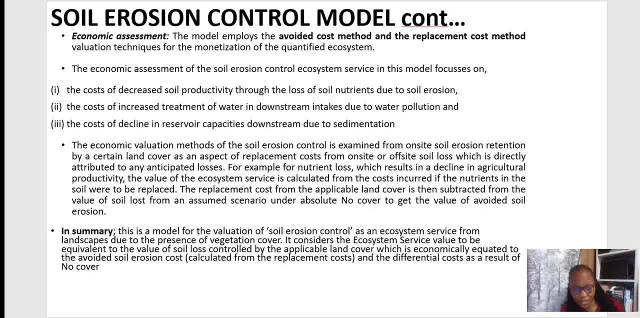 been destroyed and in most cases, you find that you have to go back to the shop to buy fertilizers to increase the soil fertility In order to replenish that soil to support crop production. So, in summary, what are we trying to say? 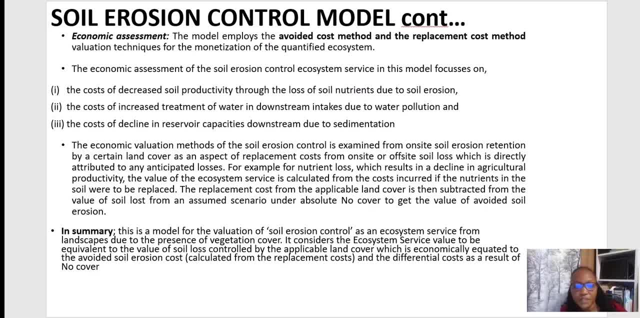 That the model for the valuation of soil erosion is an ecosystem service from landscapes due to the presence of vegetation cover. It considers ecosystem service to be equivalent to the value of soil loss controlled by applicable land cover which is economically equated. to avoid a soil erosion cost calculated from the 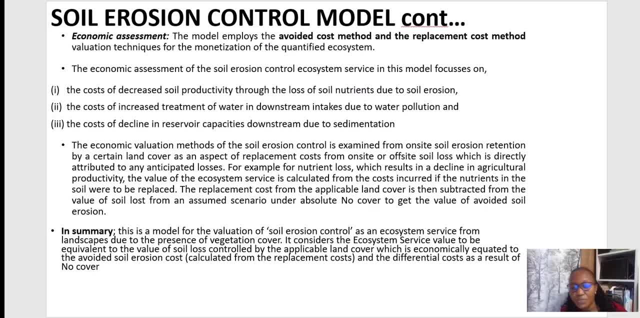 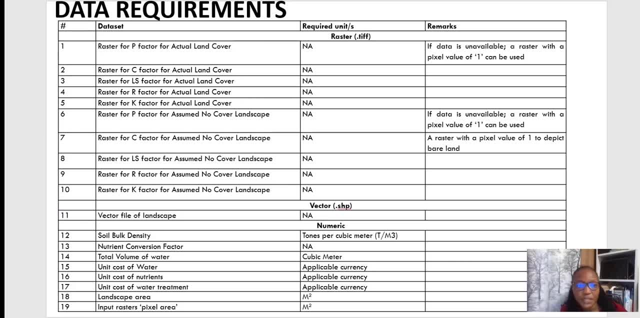 replacement cost And the differential cost as a result of no cover. What are the data requirements? There are quite a number: 19 of them. We look at the P factor. the P factor, like I've described it, the C factor, the LS factor. 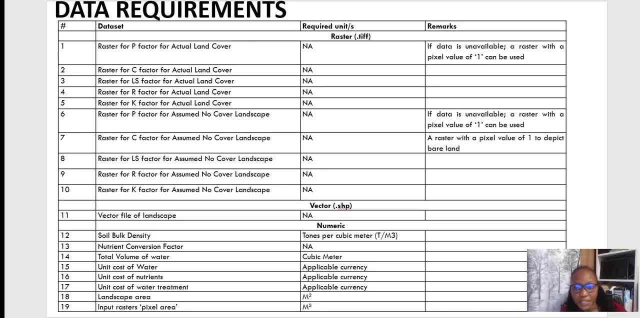 the R and the K factor and the actual land cover, be it a forest, be it a shrubland, be it a grassland. Those needs to be extracted based on the formulas that we have provided. Then we have the P, the C and the D. 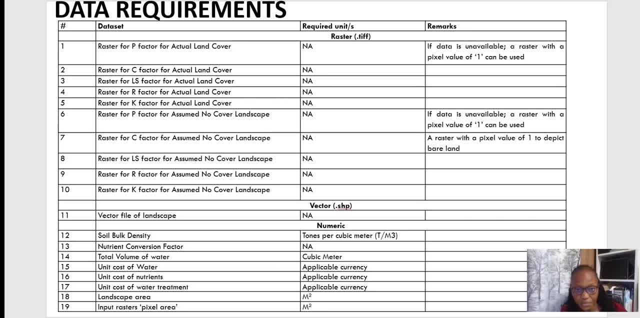 Then we have the P, the C and the D, Then we have the P, the C, the LS, the R and the K factor, which are assumed as a no cover landscape. If data is unavailable, a raster with a pixel value of one can be used. 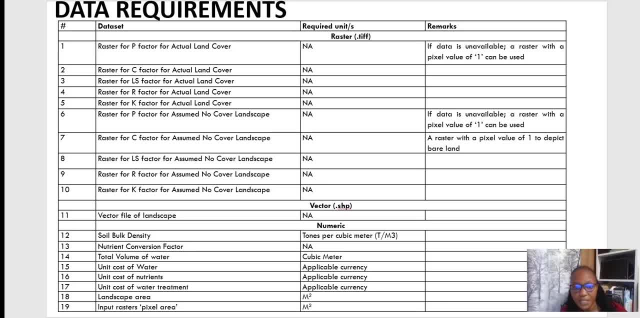 for this particular P and C factor. The rest will have to be extracted from the particular landscape under no cover. Then you need the vector file of the landscape. It's required. You need to understand the soil bulk density in terms. but you need to understand the soil bulk density in terms, but you need to have the nutrient. 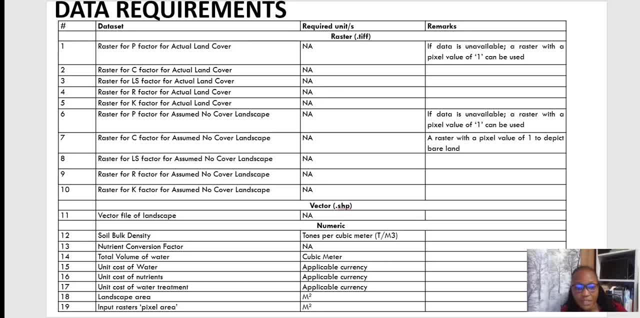 conversion factors so that you can be able to convert the soil nutrients within the soil that has been lost into the nutrients that need now to be valued based on the market price. Then you need the total volume of water that could have incurred the issues of water quality. 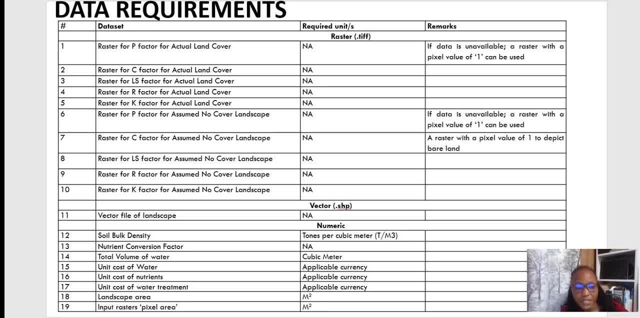 and the unit cost of that water in the applicable currency. You need the unit cost of the nutrients. Here we are saying we are comparing the nutrients in the soil, So the fertilizer is either organic or inorganic in the market. The unit cost of water treatment as a result of poor water quality. the landscape area. 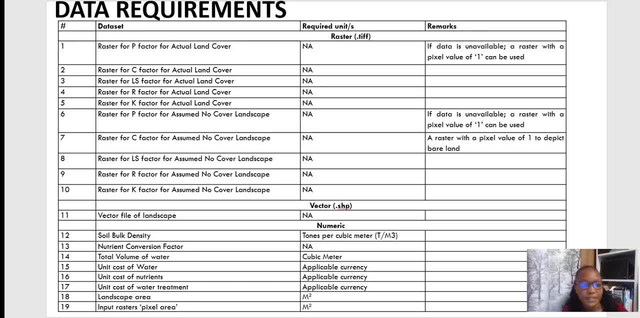 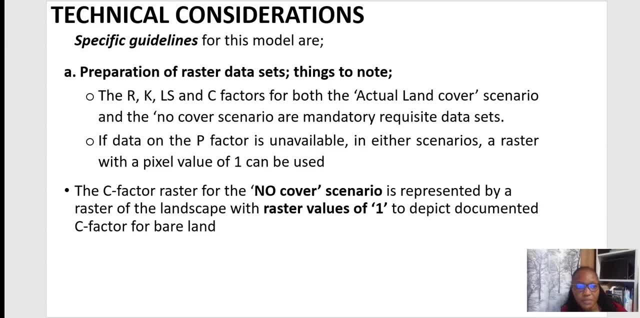 and finally, the input raster pixel areas. So what are the specific technical consideration or guidelines that you need when you're working with this model? That the R, K, LS and C factors, for both the actual land cover scenario and no cover scenario, are mandatory requisite data sets. 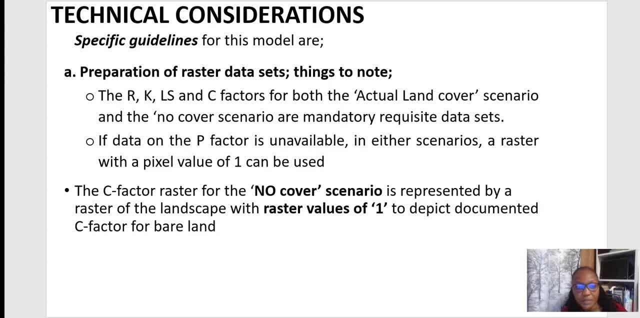 If data on the P factor is unavailable, you need to have the data on the P factor. If data on the P factor is unavailable, in either scenario, a raster with a pixel value of one can be used. We remember we said P factor is the management practices. 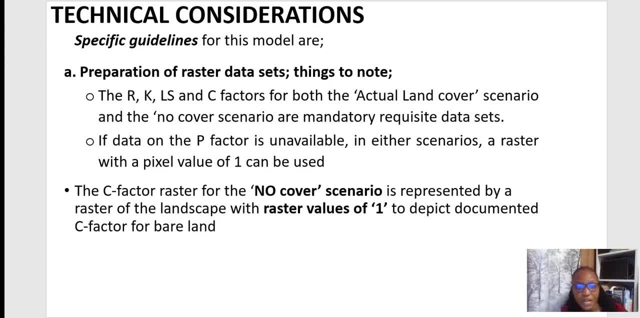 The C factor raster for the no cover scenario is represented by a raster of the landscape with a raster value of one, Because we are assuming a scenario of no cover. So if it was a forest, we are going to assume a scenario of no cover and have a C factor. 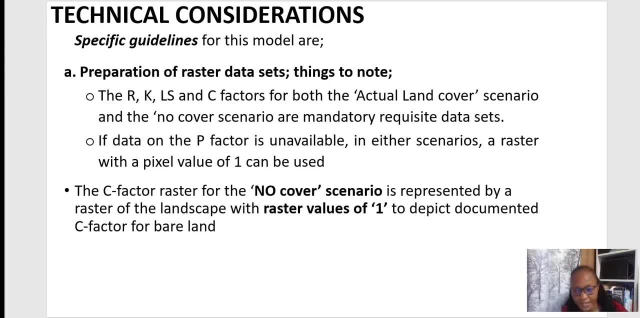 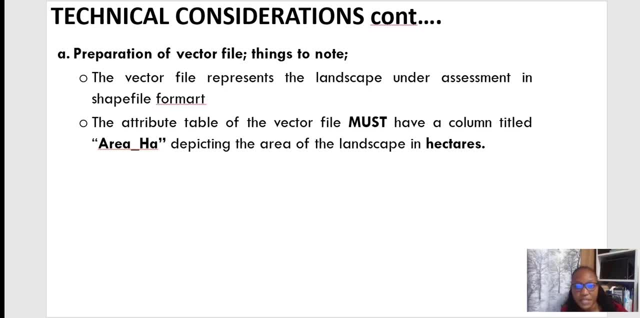 with a value of one to depict the documented C factor for bare lands. Further, in the preparation of the vector files there are things to note. The vector file represents the landscape and assessment in the shapefile format. The attribute table of the vector file must have a column titled: 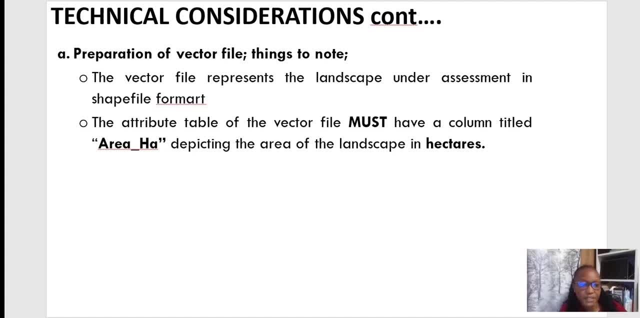 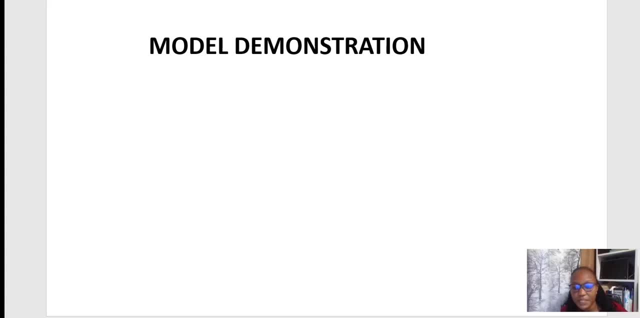 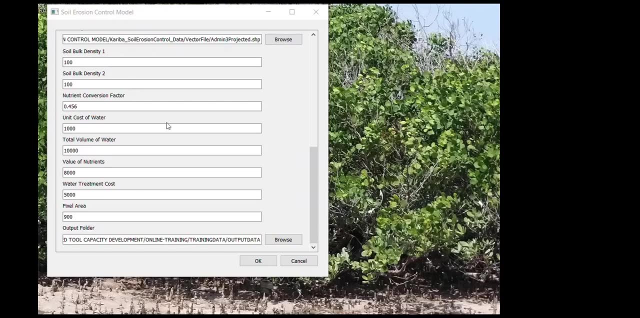 area in hectares, depicting the area of landscape in hectares. We can now finally go to the model demonstration so that we can be able to run this particular model and visualize our output. So this is how the soil erosion control model should be. When you scroll up, you can be able to see: 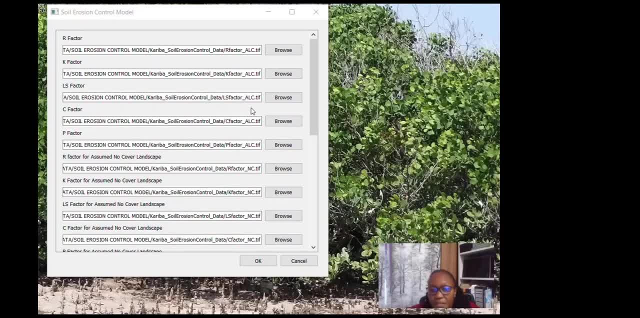 all the factors that are required to be entered. I've preloaded them because it takes quite some time loading these data sets. So we have the R factor and alternative land cover. This is the current scenario in the field. So for the first R factor, K factor, L, C and P factor is the scenario that is currently. 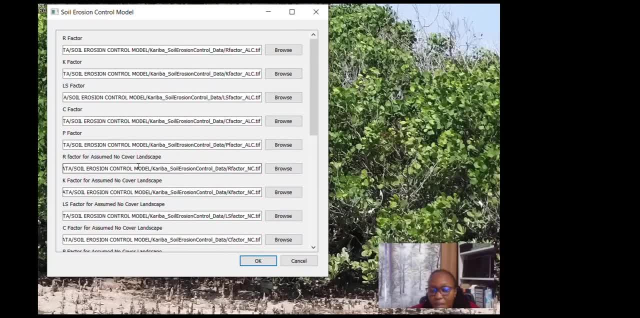 in the field, then an assumed no cover scenario, where it would be a bare land. So, for example, if the government, institution or private sector, or even the stakeholders, the local stakeholders, feel that these forests should be removed to pave way for another, bigger project that has more revenue or maybe is 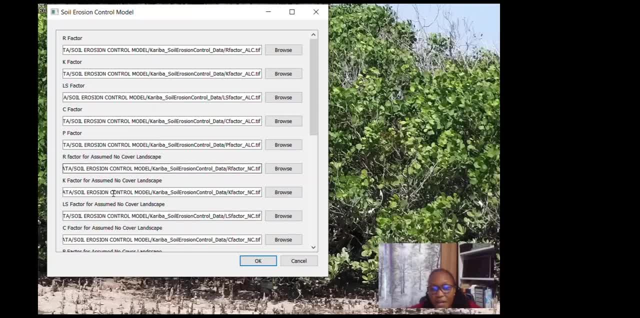 of more importance to them. then we assume a no cover landscape, because now it means whatever is replacing it. if it's not a vegetation cover, then we have to assume a bare land scenario so that we can be able to calculate and see how much soil loss will. 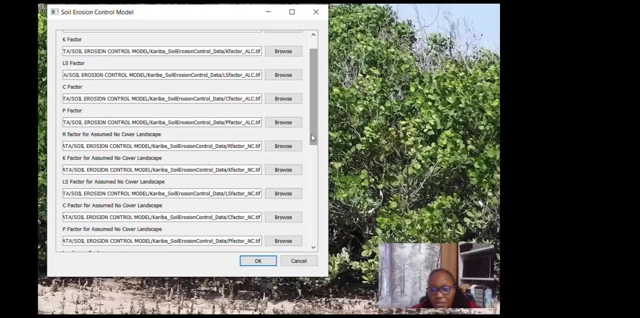 we be losing, and what is this value that we are losing as a result of converting the current land cover into something else? Alternatively, you can have where the current land cover is degraded and therefore we want to see based on the levels of degradation, whether the grasses or the forest or the shrub lands. 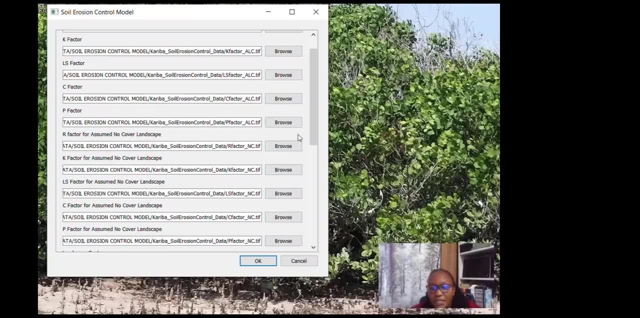 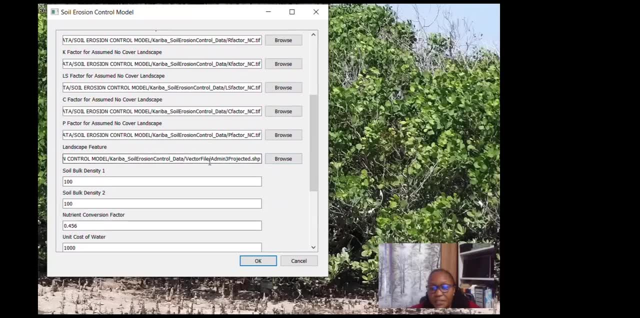 depending on how they are being depleted compared to a bare land scenario. you'd also want to see what happens. The next data set would be the landscape feature. This is a shapefile that you need to load for the landscape in question that is being 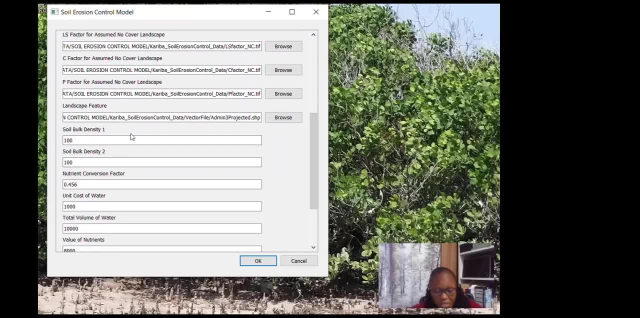 investigated for soil erosion. Then we have the soil bug density, which needs to be calculated from the field survey nutrient conversion factor. This is very key because it enables you to know the amount of nutrients that are likely to be in the soil that is being lost. 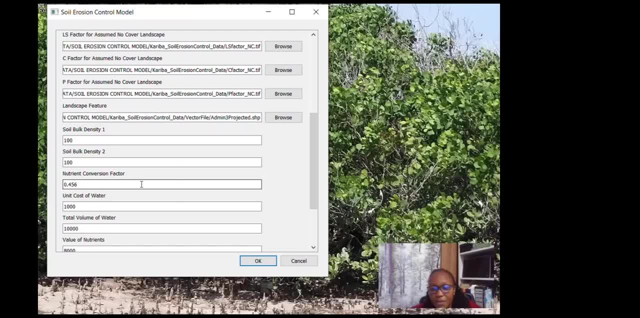 So a soil sample should be carried out to investigate the levels of NPK, Y, nitrogen, potassium and phosphorus, because the retailing fertilizers in the market usually are so high that they are not as good as the ones that are being sold in levels of NP and K. 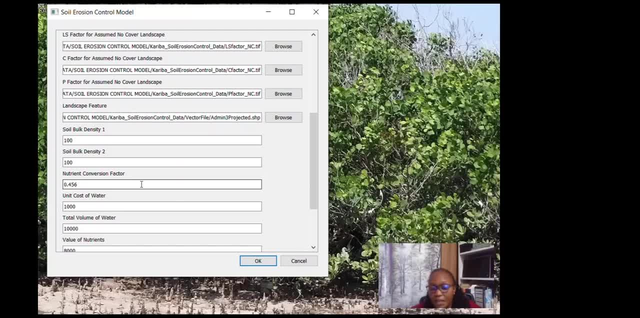 And so it's important to investigate and know how much for that small portion of soil, so that you can be able to calculate for the entire tonnage of soil that is lost, so that you can be able to account for the loss in land productivity. 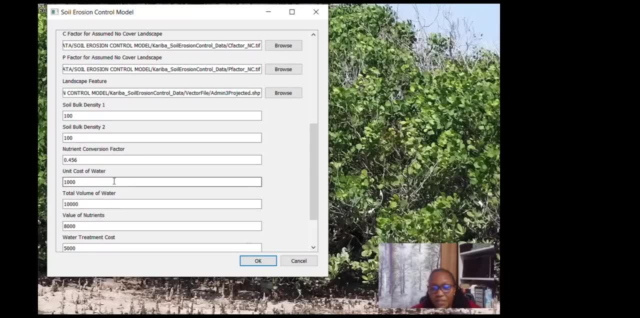 Then the next thing would be the unit cost of water. We have three aspects that we are looking at here: The land productivity, the water quality and the segmentation effects. What is the role of any land cover in terms of soil erosion control? 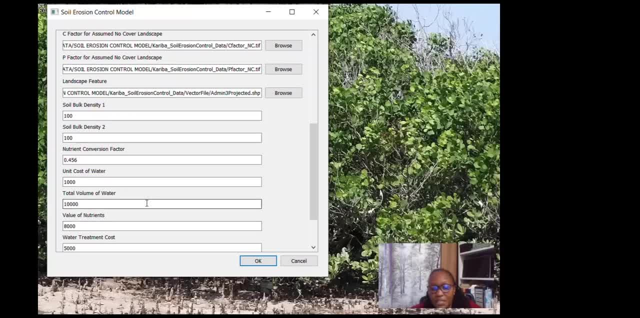 So we input the unit cost of water there and the total volume of water that is likely to have been affected by issues of soil erosion, and this has to come from the field survey, where you identify the particular water source and be able to establish the unit cost of. 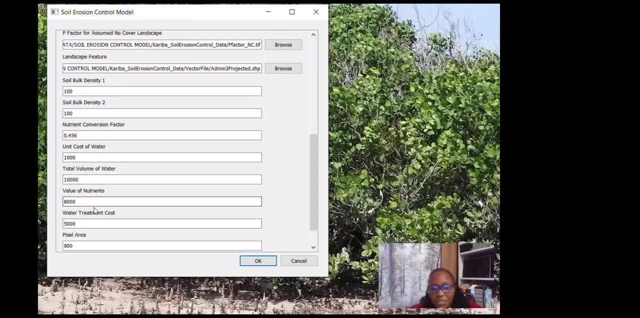 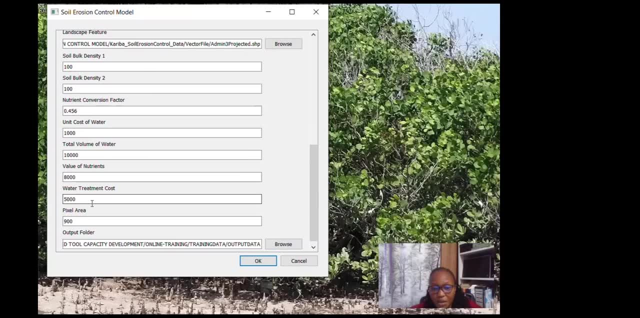 that water and the volumes that have been affected. The value of nutrients: like I've said, we are going to use the retailing market prices for the organic or inorganic fertilizers. Water treatment cost: This is the cost that has been incurred to clean this water as a result of pollution. 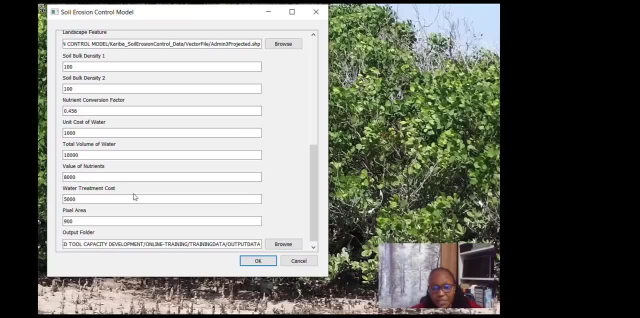 from soil erosion or as a result of segmentation. Pixel area would be based on the satellite imagery that is being used for this valuation and has been used to extract the factors that we have discussed above. And then the output folder is where you'd want to store your final output to visualize. 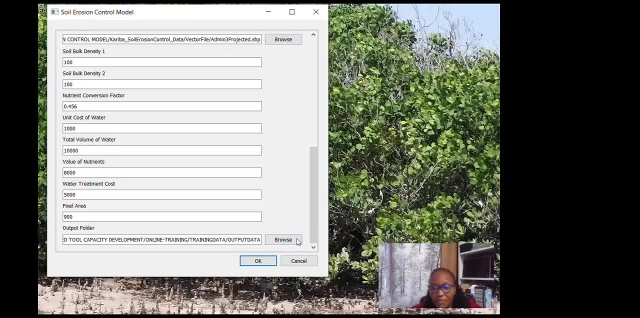 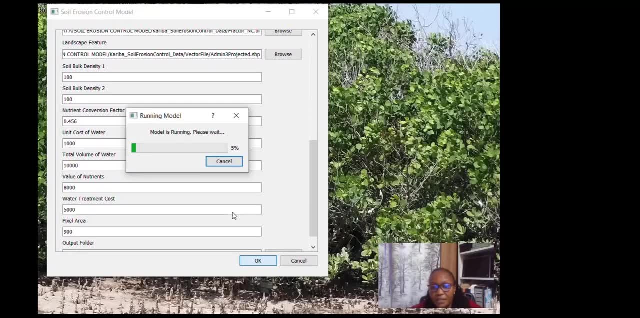 it in QGIS or ArcGIS, whatever GIS software that you have. And now that these data sets have been loaded, we'll run the model. Give it time to run. So quite a number of data inputs there. So finally, the model has finished. 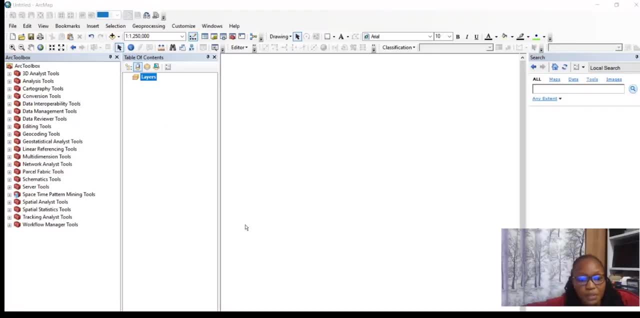 So let's visualize our soil erosion output. I will do this in ArcGIS. We can also appreciate another software. We've been using QGIS all through these lessons, So we load our data set, the soil erosion output. You can see it there. 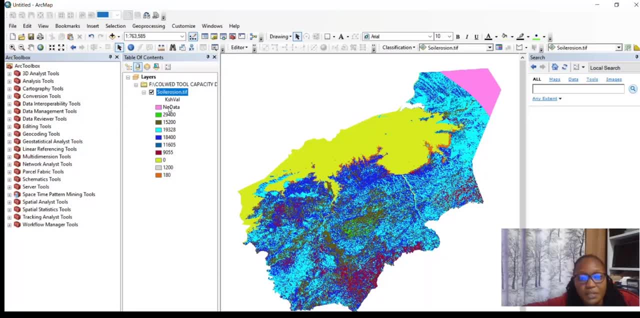 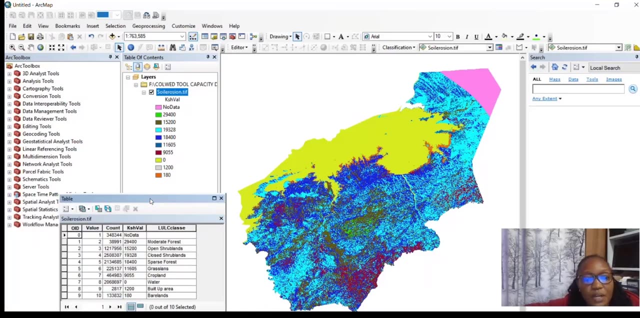 We can try to at least change the colors based on the attribute table. So the first figure there that gives us some. the first figure there that gives us some information, that shows what we have so far. So, as you can see in the model we have 22,000,. 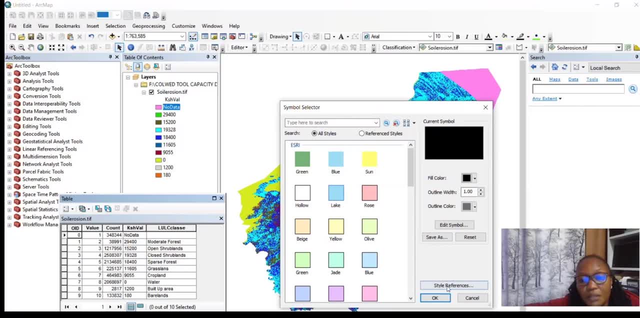 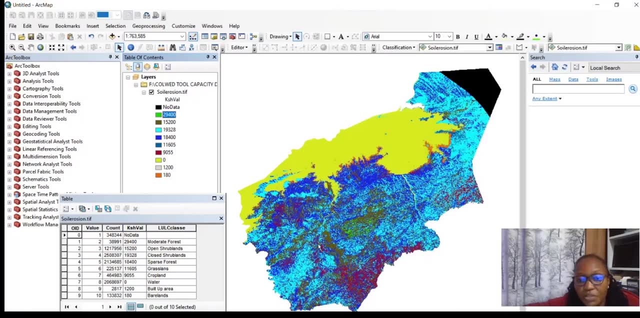 21,500 of those and 10,000, 400 is for moderate forest. We have the no data. We can put that in black because it's not within our area of assessment. So we have forest- moderate forest- in green. 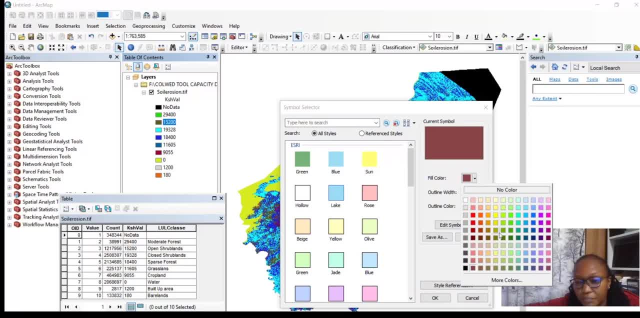 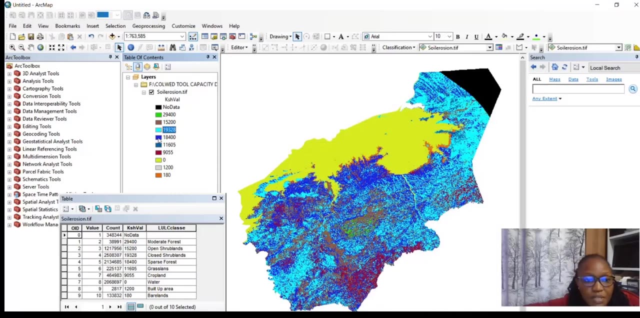 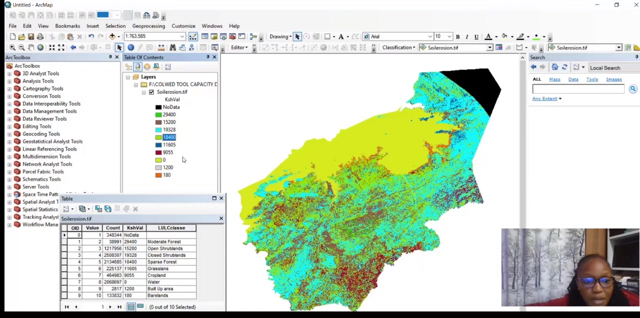 The next one is open shrubland. We can put a brown color. Oh Okay, So we have a close shrubland. it's almost similar, it's a bit lighter color. then we have sparse forest. it's a lighter green. then we have grasslands, normally in the magenta color. 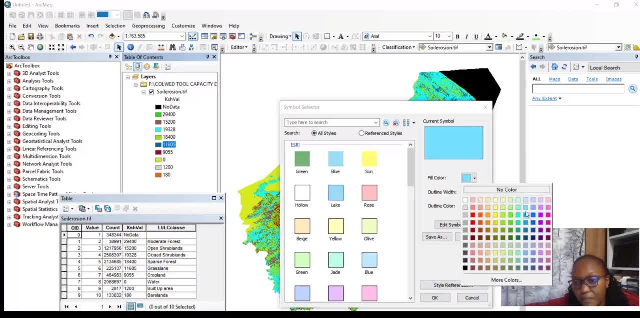 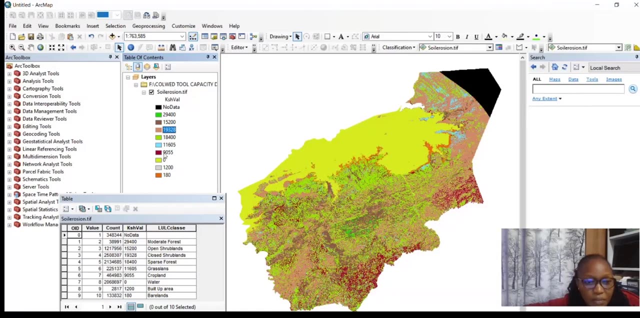 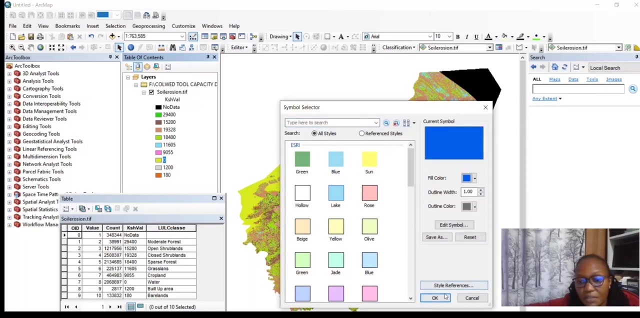 so then we have crop plant. normally the fowl uses the pink color to represent cropland. we have water. we can just visualize it in the crop plant. and then we have water. we can just visualize it in the crop land. color of water: the value is zero. it does not play any role in soil erosion. then we have the built. 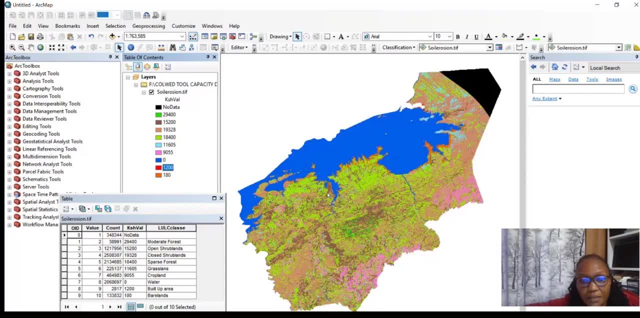 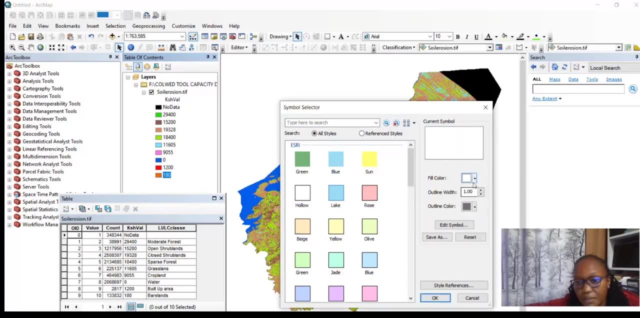 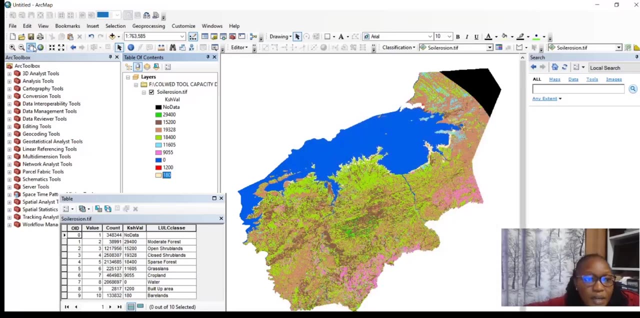 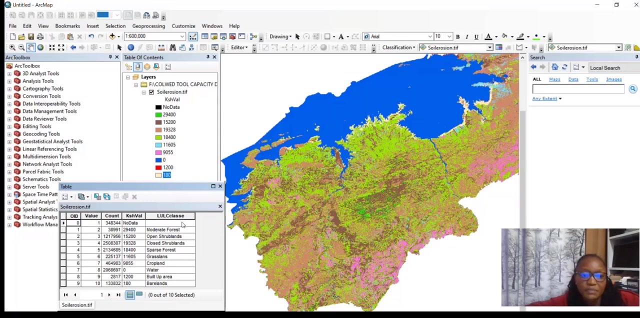 up areas normally visualized in red color, and then, finally, we have the balance. balance. we can put them in white or a color that is close to white. so we have our, we have our soil erosion output. there we can be able to see that in areas that we have moderate forest, the value is higher. 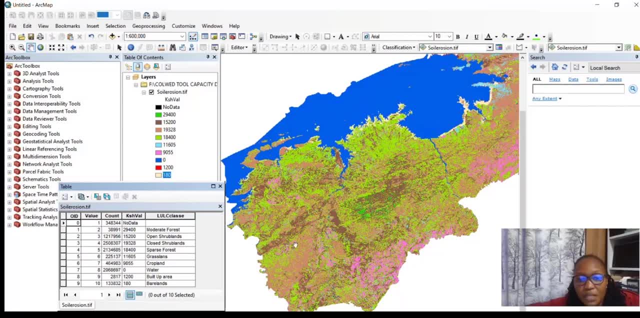 like i said, in this calculation we are looking at the tonnage of soil that is being prevented from being lost by a land cover, whether it's a forest, a shrub land or a grassland. then subtracting it from a no cover scenario, that would have a higher tonnage of soil being lost- then what we 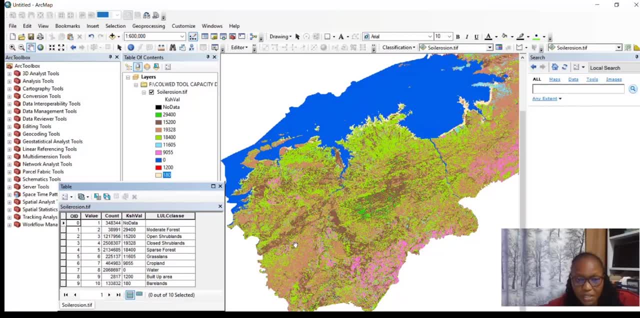 get from. the subtraction or the change that is between these two gives us what we are calling the avoided cost. that would have been cut if this soil would have been lost and affected land productivity. if soil would have been lost and affected water pollution, if there is any water source that is next to this landscape, if also. 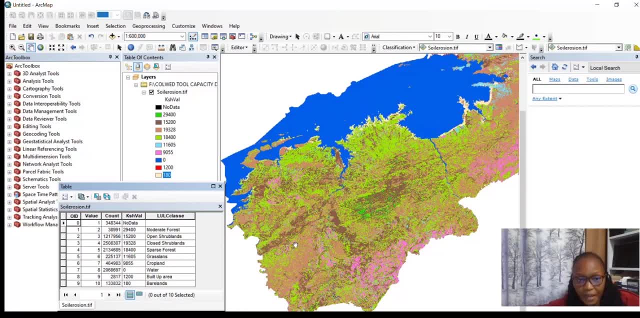 there is any issue of sedimentation as a result of the whole of this soil being lost and being moved downstream to a place where there is a wetland or even a river channel. so once we do that, then we can be able to appreciate where the soil lost is: a, for example, 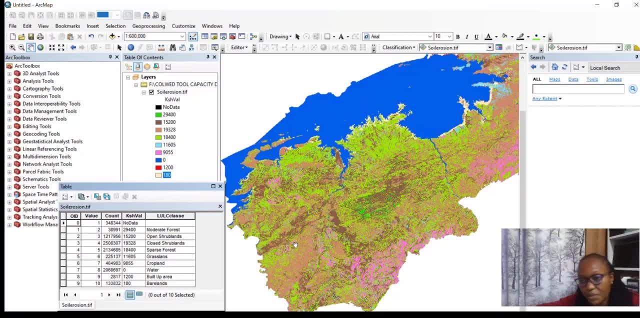 let's have a 10 000 tons of soil being lost and no cover and then under forest we have a thousand tons. that can only be lost because the movement is being slowed down by this c factor. so when you do the subtraction you realize that the soil that could have been lost as a result of no cover 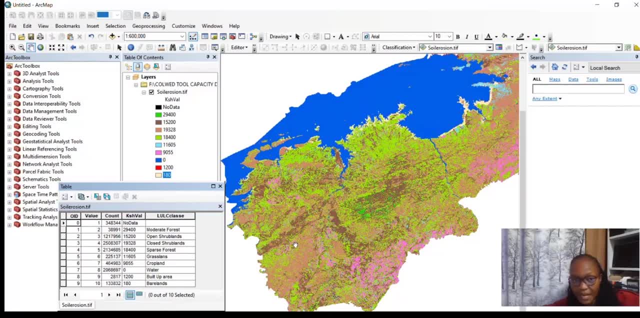 or as a result of a bare land situation, then would have been 10 000 tons minus a thousand you get around 9 000. so this now 9 000, is what we value based on land productivity. we value based on the pollution cost and treatment cost of water and we value based on the treatment cost as a result of. 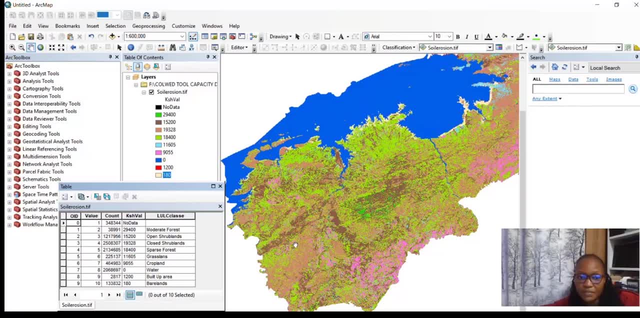 sedimentation. so you find, for forest, moderate forest, the value is high. for the grasslands, the shrublands, the sparse forests, you realize the the, the values are significantly higher because they play a very key role in reducing soil erosion. and that is it from us for today. we welcome any questions and answer. 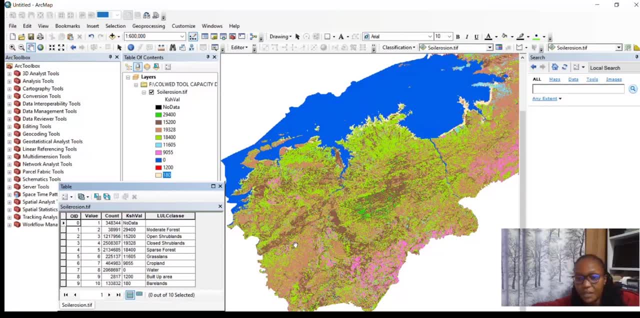 sessions on the three models that we have discussed today. all our models are basically, uh, almost a hundred percent the process based: the soil erosion, the water storage and the terrestrial product. let us have key discussions to see whether any areas we can improve. uh, what do these kind of statistics say in book, for example, when 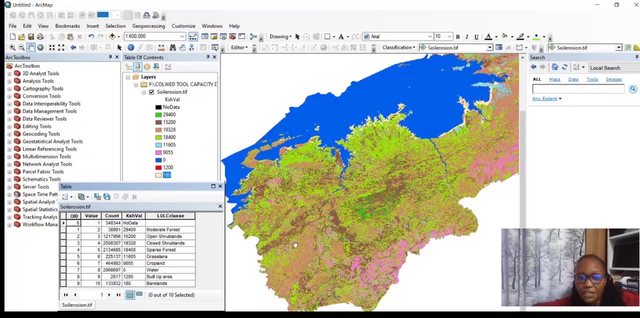 you look at the soil erosion, the key statistics here in book- that vegetation cover is very important. others, if you have scenarios of bare land and built up areas, possibilities of losing higher soil erosion. possibilities of having a clogging of drainage systems, sedimentation of water sources, loss of land productivity. that is key not only for cropland but 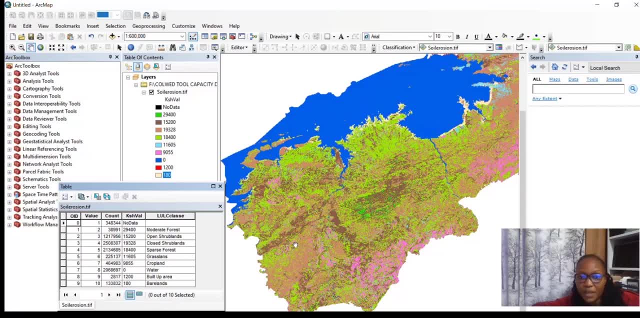 also for biodiversity. So those kind of statistics are those that you sit down with key decision makers to tell them if they're planning to actually remove a very significant ecosystem that plays all these significant ecosystem functions that lead to significant ecosystem services. then you can be able to see how operating under this ecosystem- because there's a 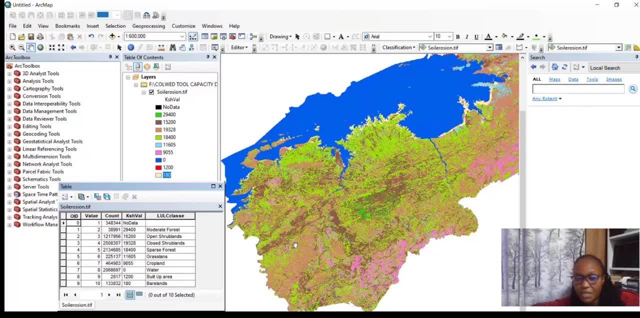 very important need, very important economic need. how it can be done. What are the trade-offs that can be done? Because land degradation neutrality under UNCCD calls for trade-offs so that we can be able to utilize our ecosystems sustainably. We may want to protect, but at times when we protect, 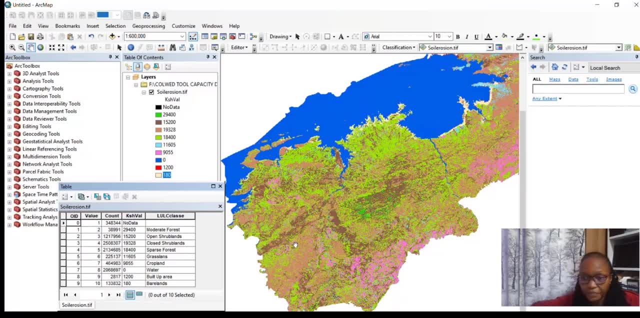